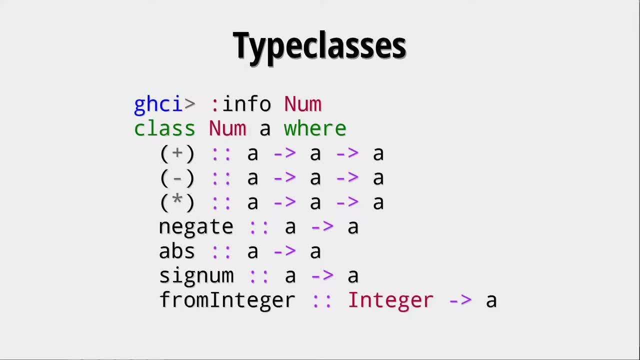 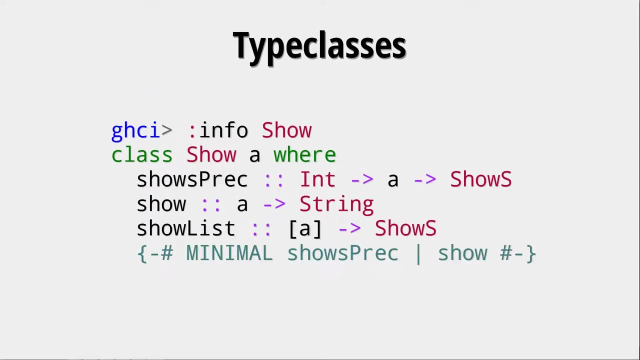 this type class. So, for example, plus minus multiplication negate absolute signum, which gives you a representation, So you can get a representation of the sign of this number and from integer. Okay, So maybe let's look at other type classes that are really interesting, like show. 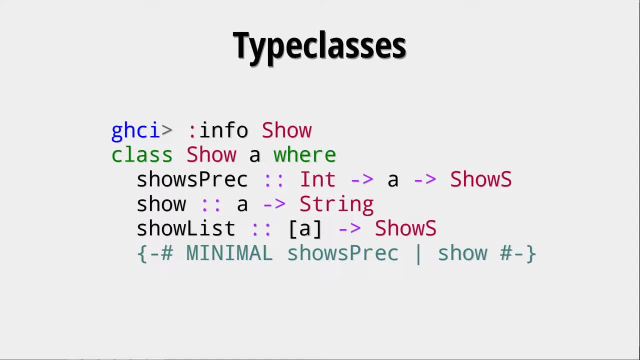 If you want to print a type in ghci, for example by just typing out this type, it has to have an instance of the show type class. Here we see something else which is interesting. We have this minimal showsPrag and show. What does that tell us? 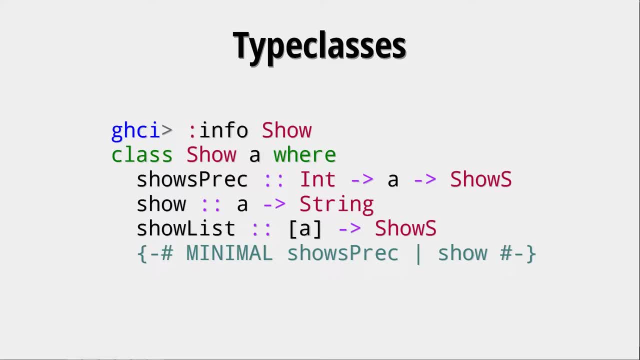 Well, This tells us that we do not need to create all of the functions that we see here, all of the three. We actually only need to create either showsPrag or show, And if we have one of these functions, all the other functions are implied. 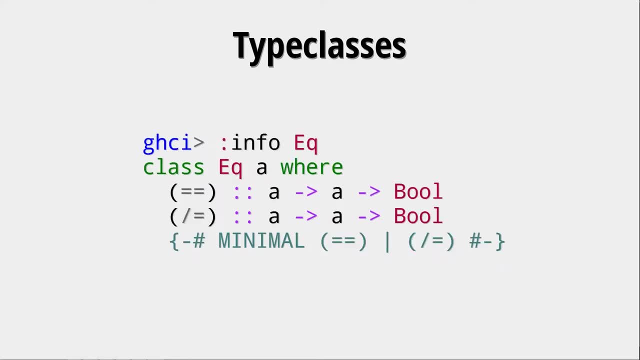 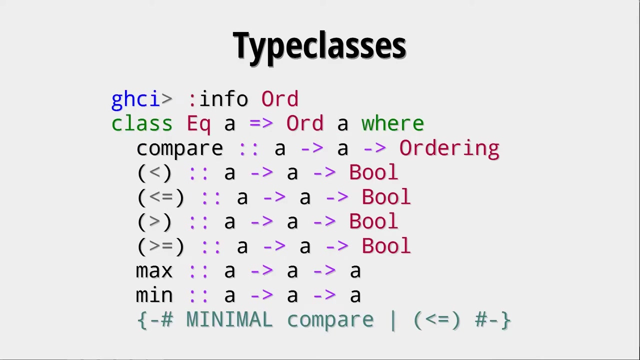 That's a point where Haskell can then derive the other functions from, Just like here in this eqType class, where we have types that can be tested on equivalents. here we only need to define equals or not equals, and of course the other function then is derived from the Boolean inversion of the other function. 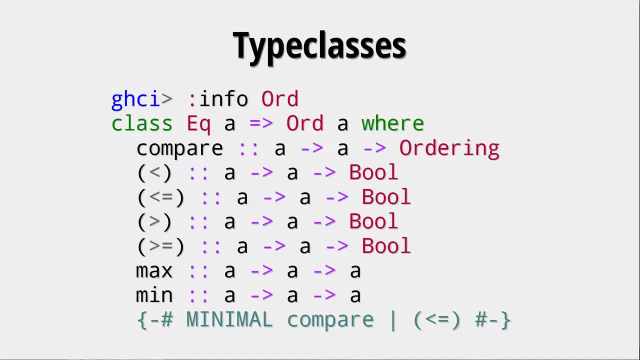 Another important type class is ord, where we have some ordering. By the way, what we can see here is that eq implies ord or it doesn't really imply ord. It's the other way around. So in order for a type to be in the ord type class, 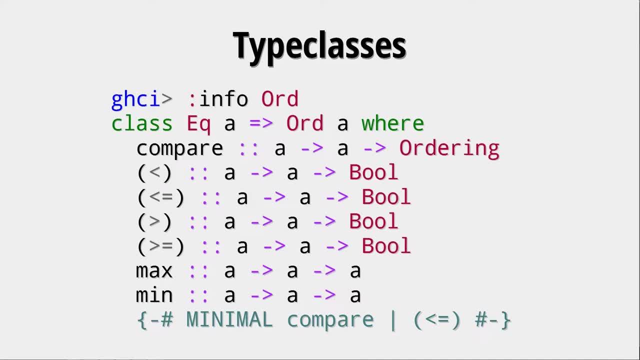 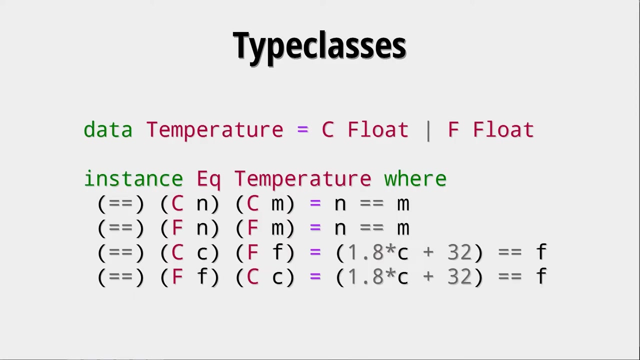 It also needs to be in the eqType class, So everything that can be ordered can also be checked for equivalents. And here we see that the minimal type class that we need to give is either the smaller equals or the compare function. So let's look at an example how to do such an instance of a type class. 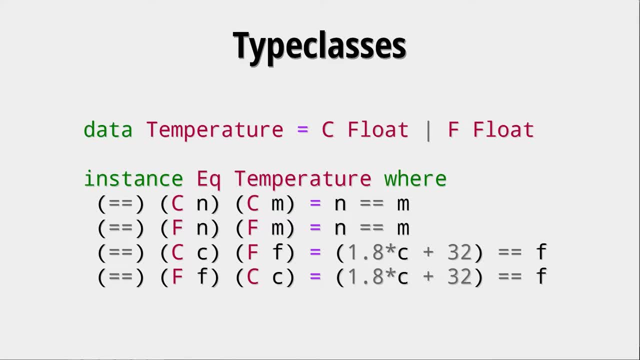 So here we have a data type temperature, Which stores temperature either in Celsius or Fahrenheit. So that's a bit of a problem, Because how do we compare that? Well, we create an instance of the eqType class for this temperature, And here we see that the not equals is not defined. 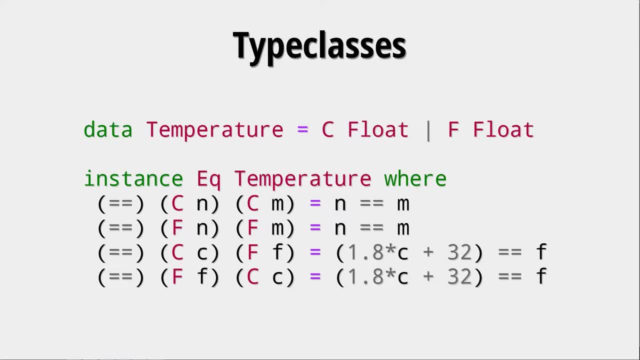 It's derived implicitly. We only define the equals. And that's the point where we well, if we have two Celsius temperatures, we compare them, If we have two Fahrenheit's, we compare them, And if we have some mixed temperatures, then we do some conversion and check that for equivalents. 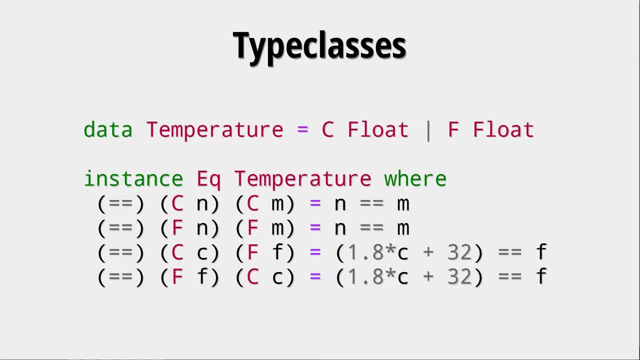 By the way, this will probably not work correctly because floats are not that precise in Haskell. So this 1.8 times c will probably have some rounding issues. But that's not that important here. The important thing here is how to define such an instance of a type class. 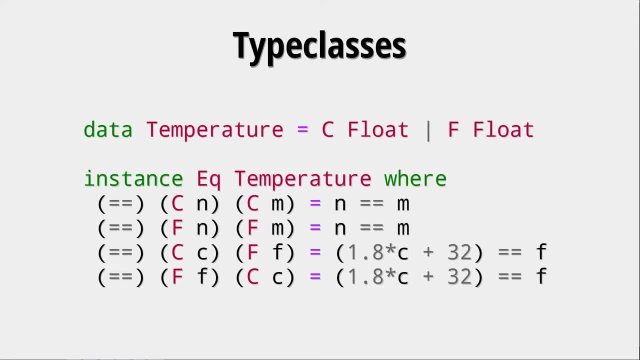 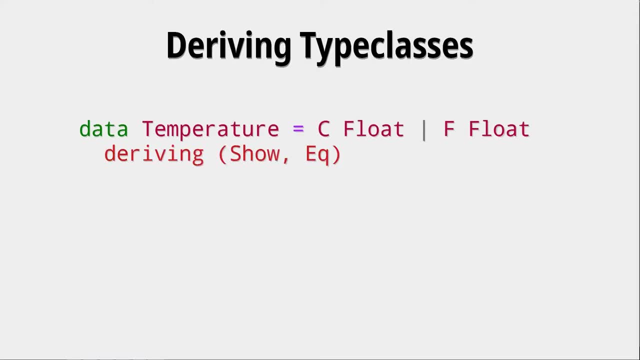 And, of course, if we wanted temperature to, for example, be in the numType class, we would have needed to define much more functions, But that always depends on your use case. So what you can sometimes see and do is this: deriving And deriving type classes can be well, very beneficial. 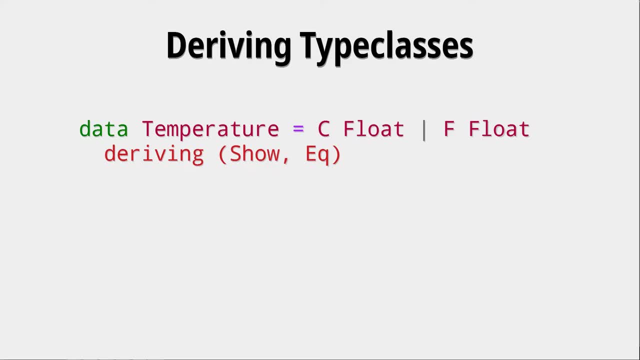 For example, if you want your data types to be printable, you don't want to write new instances of the showType As all the time. that would be well. that would be a bit of a waste of a time. So we can do this deriving: 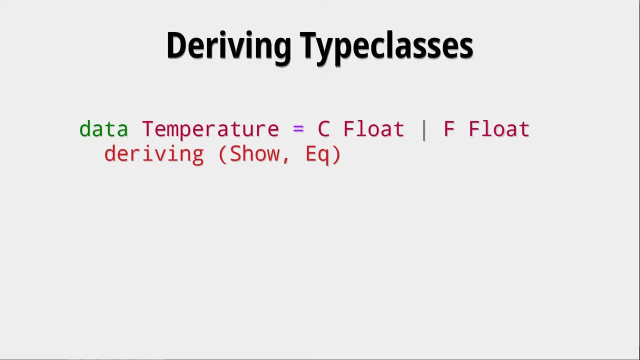 And deriving means that Haskell has to figure out how to create an instance of this type class for this type. So with show this is, I think, always possible if you use types that have an instance of the showType class And how it does. that is that in the end. 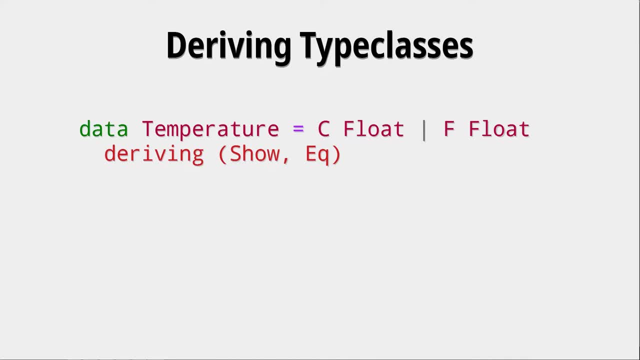 printed type just looks like the type you would type it in in Haskell. Now, with the EQ, this is a bit different, because we just seen how to correctly define the equivalence for this temperature type. The question is: how does this deriving EQ actually derive the equivalence? Well, it doesn't do it. 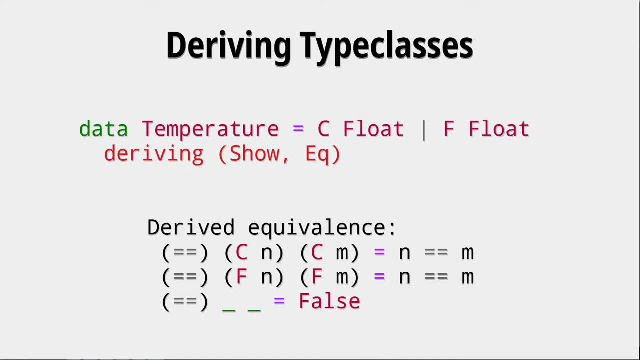 correctly. The derived equivalence does the following: It compares if the constructors are the same, and if they are, it compares whether all the arguments for the constructors are the same. This is structural equivalence, because it looks at the structure of the data type and checks if.